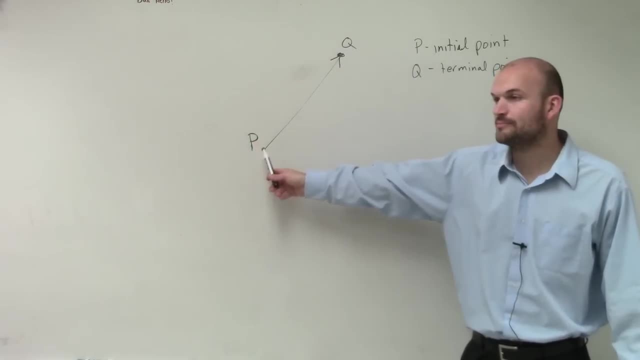 from Q to P, right in this example. So we're going from P to Q, So the direction of the line segment matters, right, or of their directional line, And then also we need to look at the distance, right. So those are going to be two things that we're going to talk about. 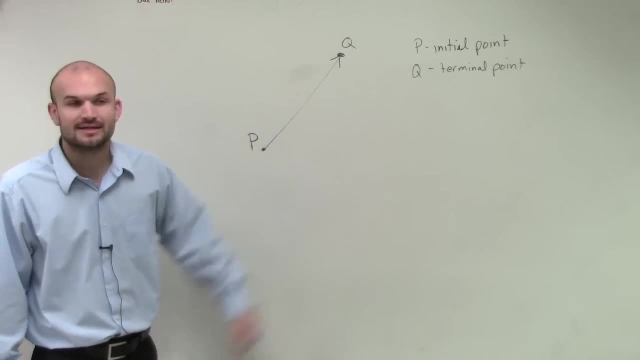 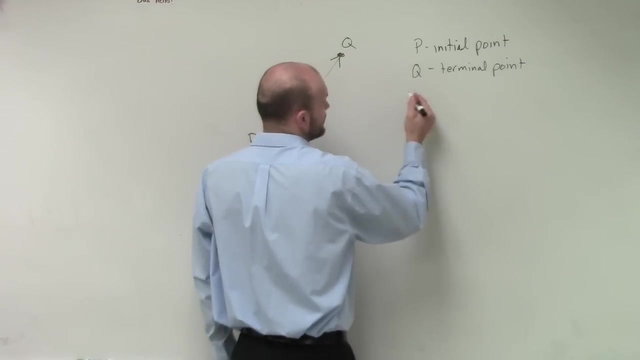 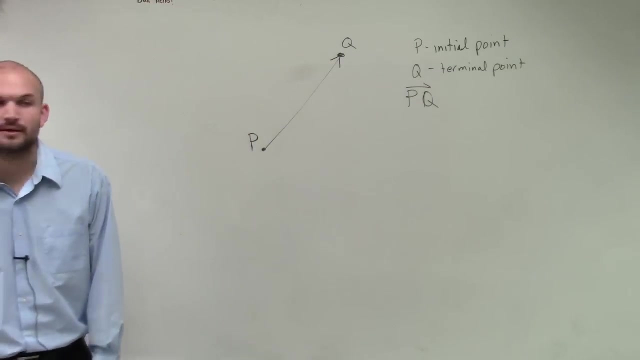 And when we have a directional line segment in a plane, a lot of times what we're going to call them is a vector. So first of all, we can say that if we go from P to Q, we can write this as P to Q is going to be your line segment. All right, And now, a lot of times, 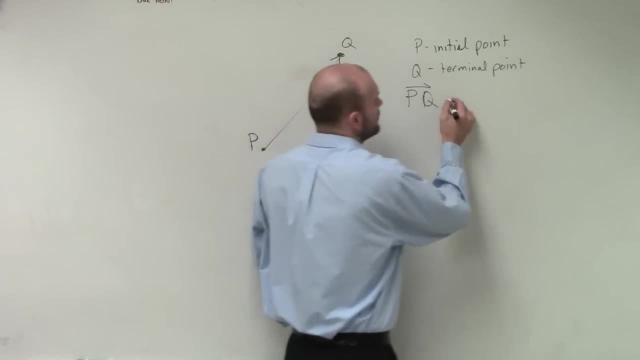 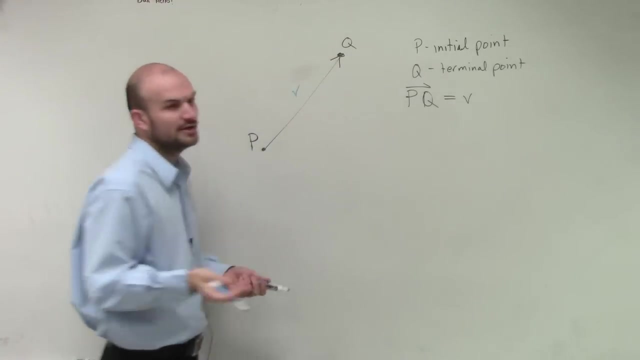 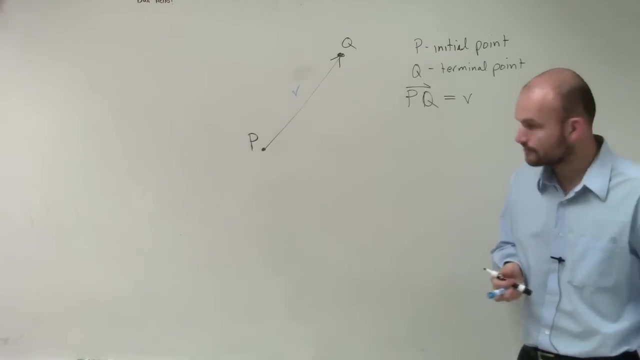 what we do is when we have a directional line segment on a plane, we give them kind of lowercase letters which would be like a vector V, And you could call them vector U, vector V, vector W. Those are kind of more of our common terms for our vectors. So what's important then? 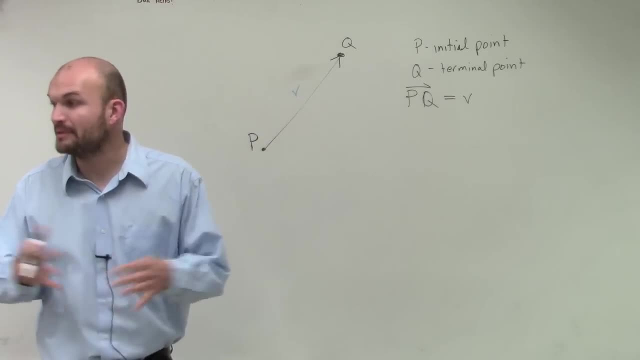 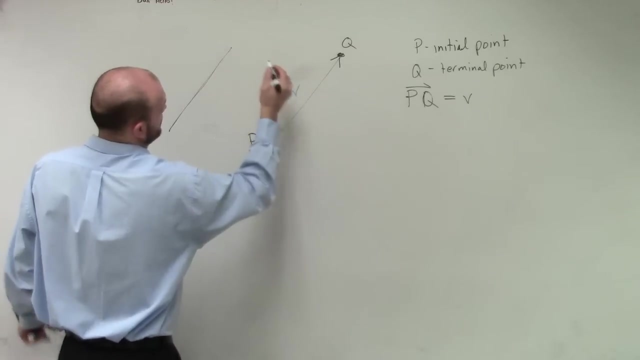 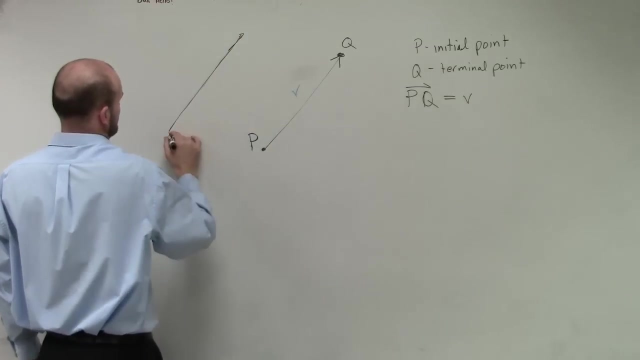 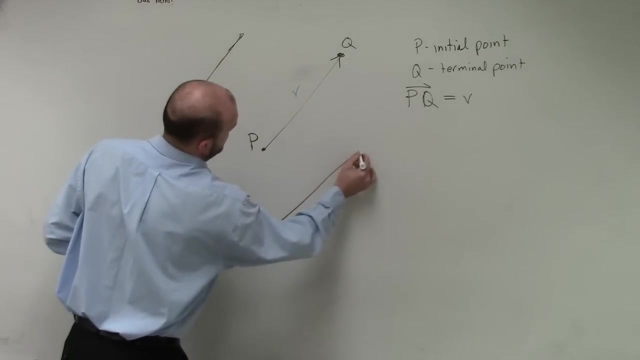 is if we're looking at one vector and we want to kind of maybe compare it to some other vectors and rather than just kind of going with the terminal points here. let's say, I have one vector here, What's wrong with my marker? All right, I'm going to do my best. I understand. 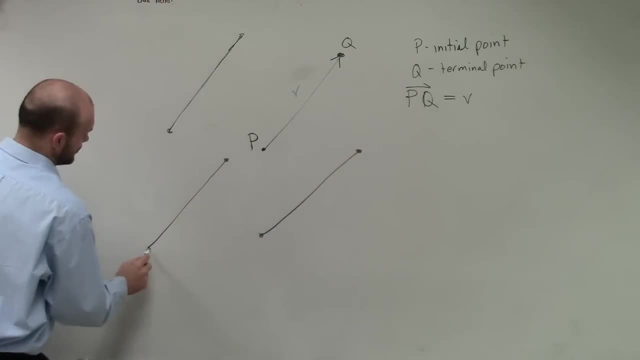 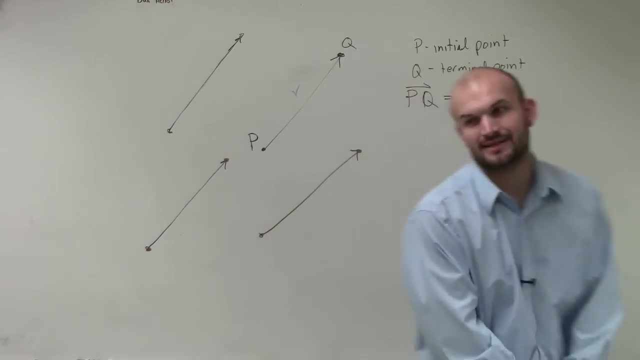 that these don't all look exactly the same. But, if you guys can see, what I try to do is I try to create the same slope with each one of those vectors And I also try to create the exact same distance or length of each one of those. 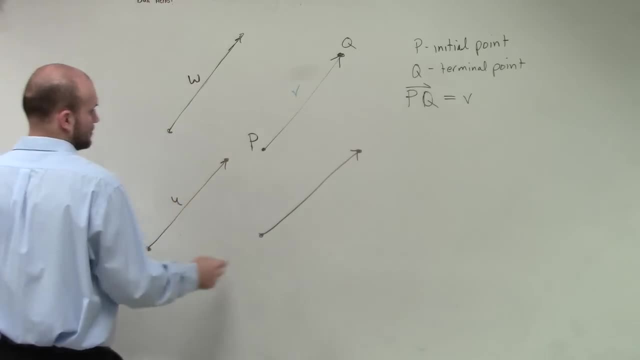 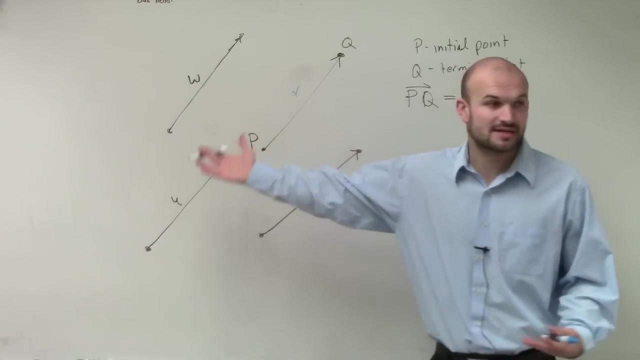 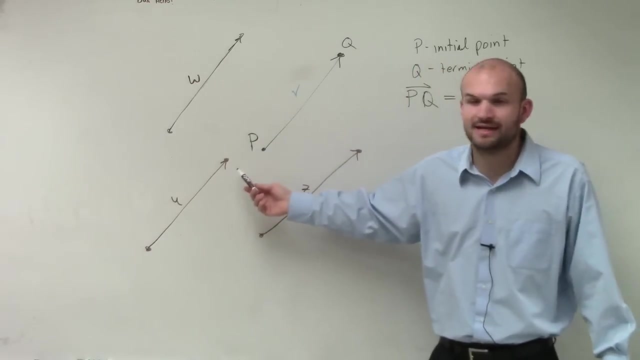 All right. So one thing I want you guys to understand is when talking about vectors, all right, they're vectors on a plane, As long as they have the same direction slope and they have the same magnitude, which is going to be our distance, which we'll talk. 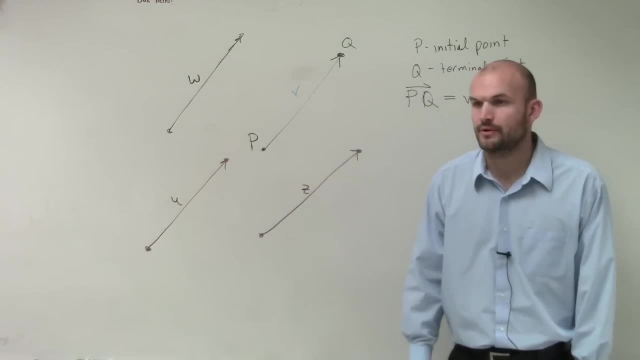 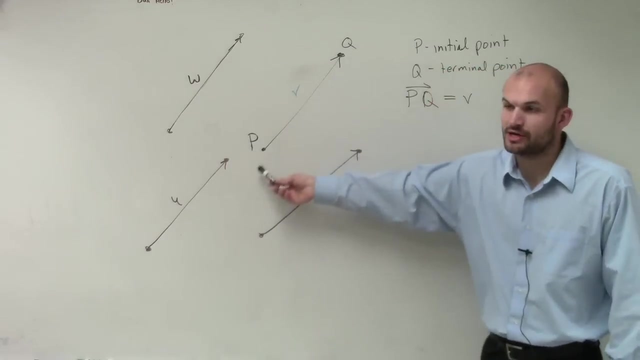 about in a second. then they're all going to be equal to each other. Okay, Everybody make sense of that A lot of times. yes, we can call a directional line segment from our initial to our terminal. We can write it like that, But more commonly, the way that.